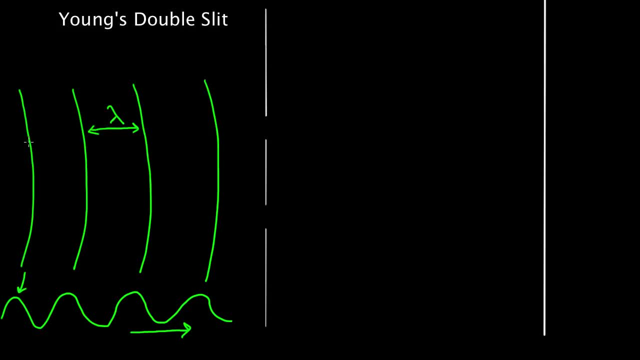 This represents a peak. Everywhere along here is a peak of the wave. So you've got this wave filling up this entire region. These lines represent lines where every point along there is a peak of the wave. What's in the middle, Yep? 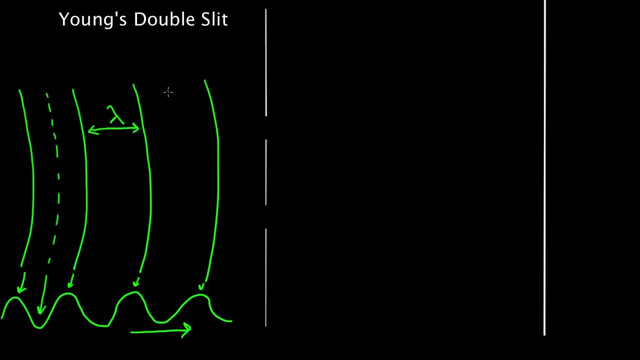 In the middle would be the trough of the wave or the valley. So that's what I'm going to use. I'm going to use this representation for the wave. This will let me show this wave spreading out in two dimensions better than this one could. 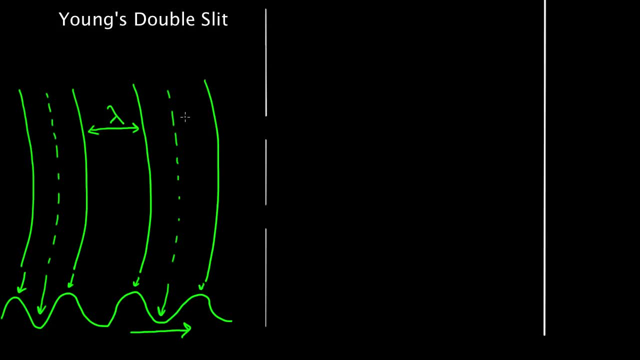 I couldn't draw it very well with this one. So what happens? This wave comes in here, This laser light comes in here. Well, that part hits that barrier, It doesn't get through. This part hits that barrier, It doesn't get through. 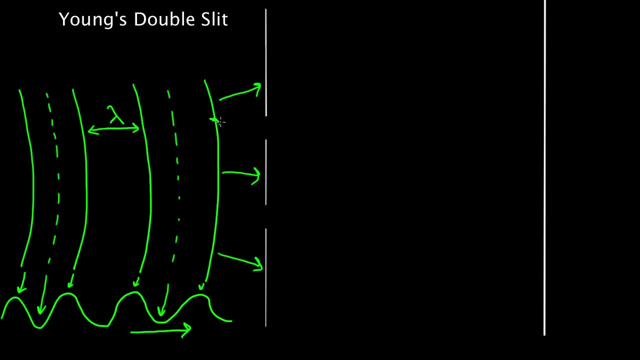 This part hits the barrier. It doesn't get through. The only portion that's going to get through is basically this portion here and this portion here. These are going to be the ones that make it through, And so what happens? What do you see on the wall over here? 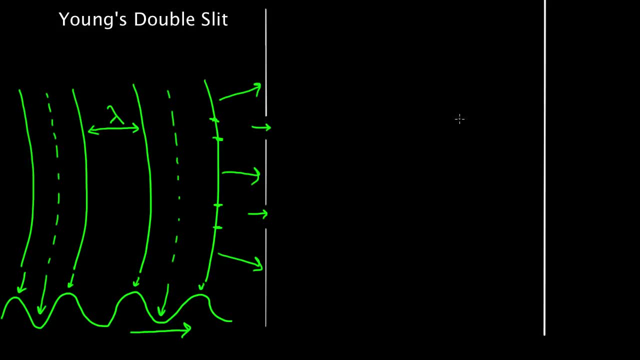 If this was a screen that you could project the light on, what would you see? Well, naively, what I would have thought I'd have been like: okay, shoot, light comes through here, bright spot. Light comes through here, bright spot. 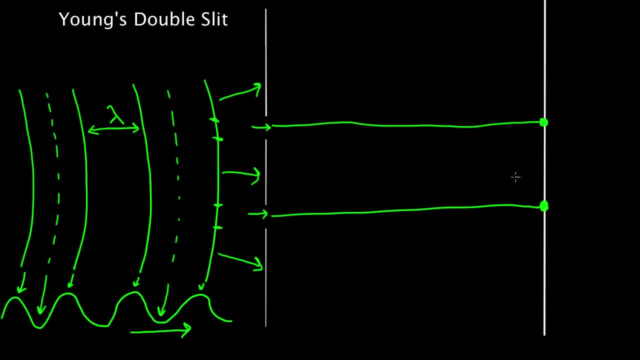 You just get two bright spots, right. Well, no, that's not what you get. That's why this experiment is interesting, because you don't just get two bright spots, You get a pattern over here, because waves don't just travel straight through this hole. 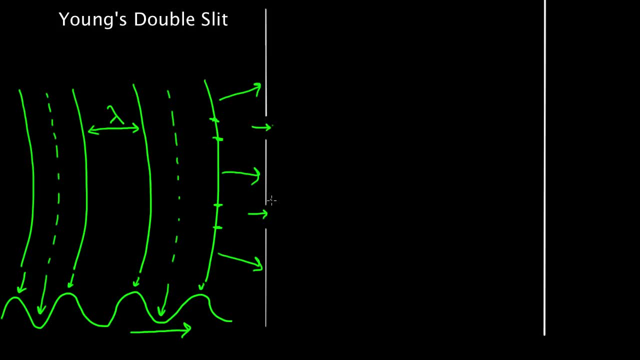 When a wave encounters a hole or a corner, it spreads out, and that spreading out we call diffraction. So you're going to get a wave spreading out from down here. It's not going to go in a straight line. It spreads out in two dimensions. 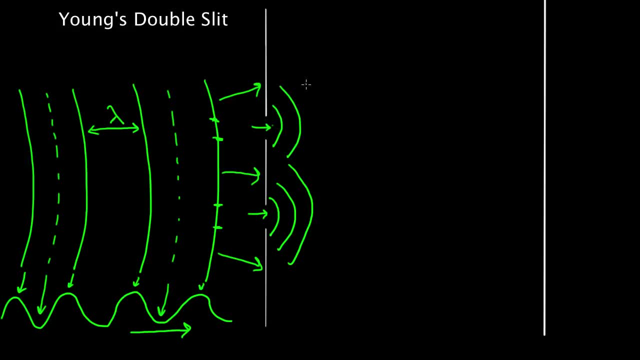 That's why I had to use this wave drawing representation. It's going to spread out from the top one too. Uh-oh, look what's going to happen. You're going to have two waves overlapping. These two waves are going to start overlapping. 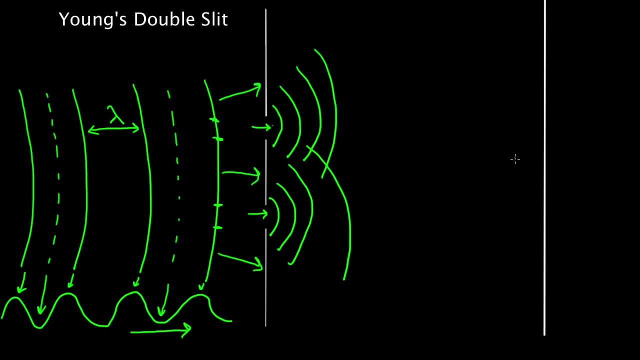 and where they overlap constructively, you'd get a bright spot. Where they overlap destructively, you'd get a dark spot. Where it's sort of half constructive, half destructive, you might get a mediumly bright spot. How do we figure out what's going to be? 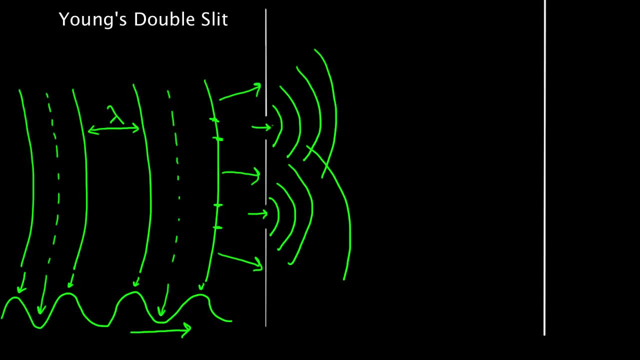 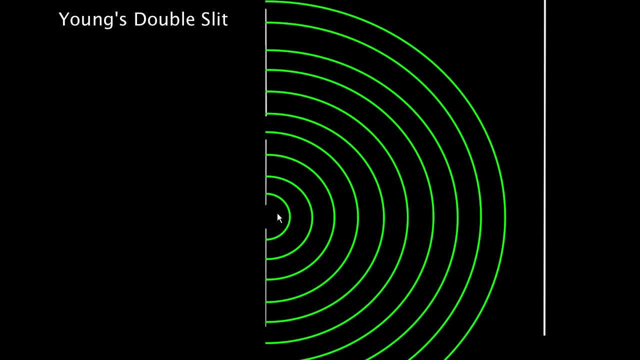 Well, I can't draw this precise enough to show you that. So let me get rid of all of this mess real quick. Get rid of that Out of the bottom hole. what would you get? You'd get this, a nice spherical pattern, coming out of here. 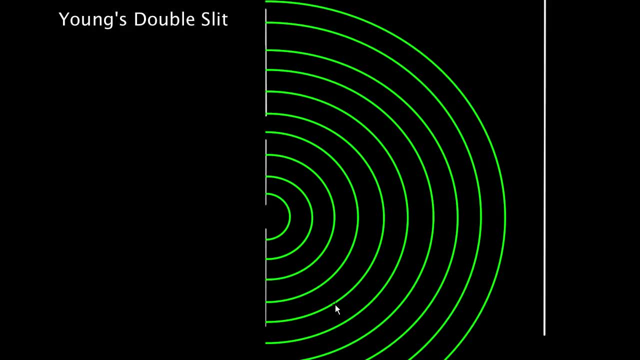 Now it might not exactly be the same intensity throughout here, but I can't draw it with the exact right intensity up here. This intensity of this portion would be smaller than this portion here, the degree to which it's spreading, But this will help me visualize it. 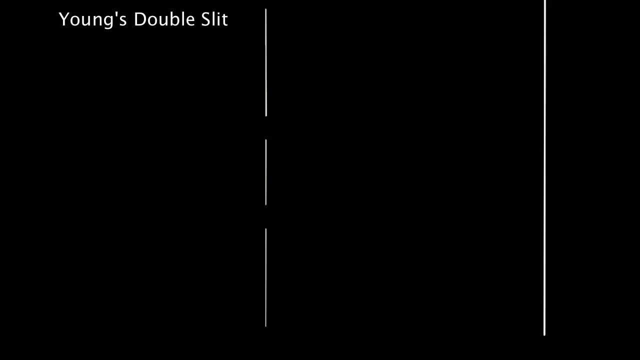 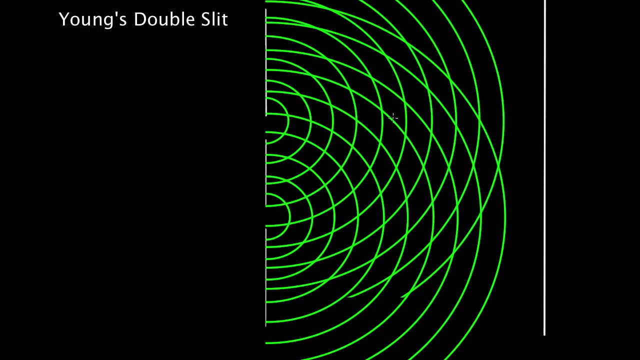 You've got this wave spreading out out of the bottom hole. You also have a wave spreading out of the top hole And now these are going to overlap. Let's draw them both: Boom Waves overlapping in the same region. You're going to have constructive and destructive interference. 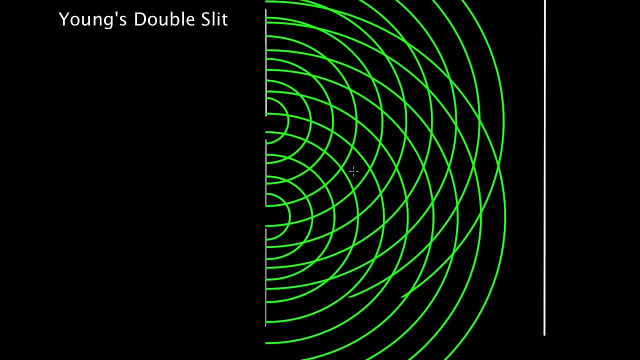 And if you look, remember these lines represent peaks. So every time a peak lines up right over a peak, or in the middle, a valley over a valley, every time the wave is exactly in phase when it gets to the same point. 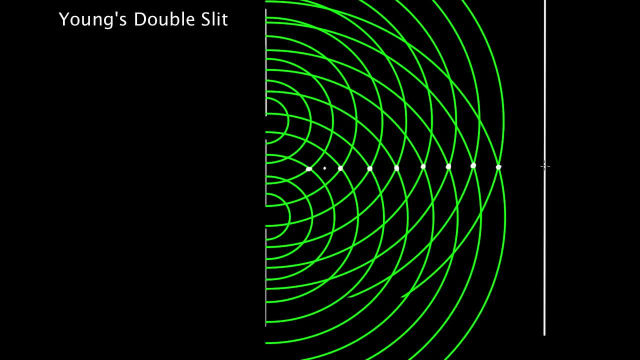 these are all constructive points. So right in the middle you'd get a big bright spot. That's kind of weird. Right in between these holes there'd be a big bright spot. Where else? Well, look at this Right. 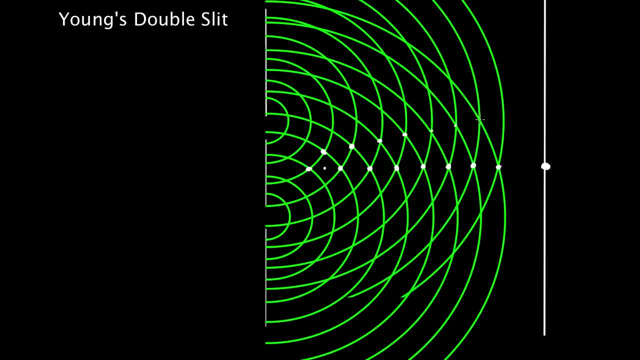 This is constructive, Constructive, all constructive. They form a line, They get these lines of constructive interference Same with this line: Constructive, Constructive, all the way over to here. So on the wall you'd see multiple bright spots down here. 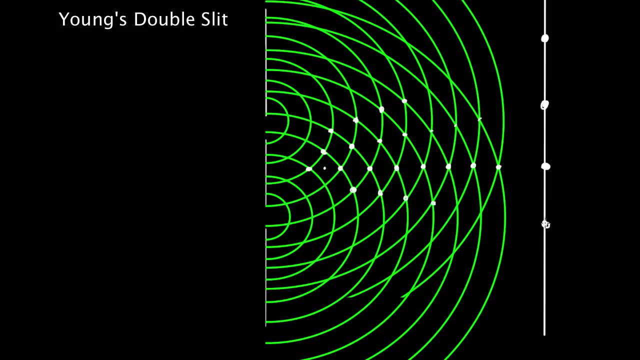 These are all constructive because peaks are lining up perfectly. And I'd get another one here. You keep getting these bright spots on the wall. They wouldn't last forever. I mean at some point it'd start to die off. It'd be hard to see. 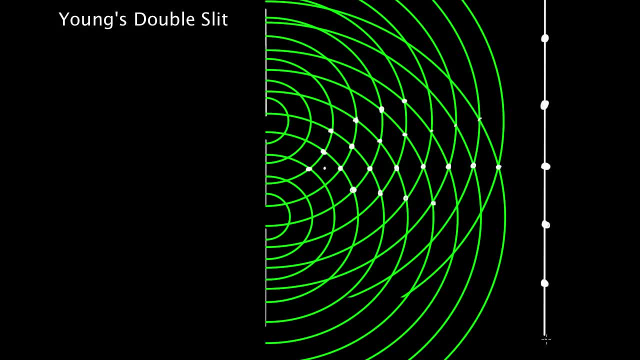 But you'd be getting these bright spots continuing on At some point. they're so dim you can't see them. And in the middle, well, wherever Let's see What's a good point to look at? Wherever a peak lines up with a valley. 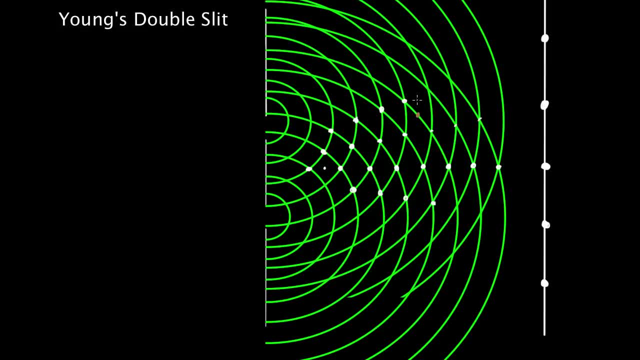 So this wave's a peak right here. But for the other wave, look it, We're in between the two green lines. So at that point you'll have destructive, because the peak is matching up with the valley And this would be destructive, and this would be destructive. 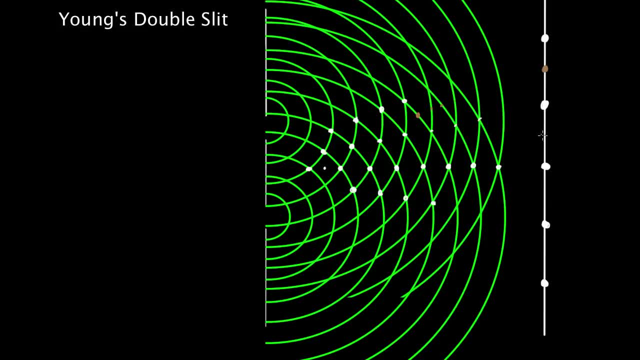 So in between here you'd get a destructive point. The same is true In between each of these perfectly constructive points, you'd get a perfectly destructive point In between those. it'd be kind of half constructive, half destructive. It'd merge into each other. 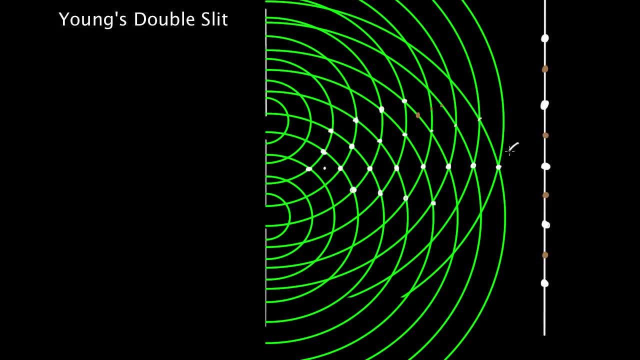 And what you'd get. sometimes, physicists draw a little graph to represent this. You get a bright spot in the middle- This is sort of representing a graph of the intensity 0, and then another bright spot, And then it goes down to 0. again another bright spot. 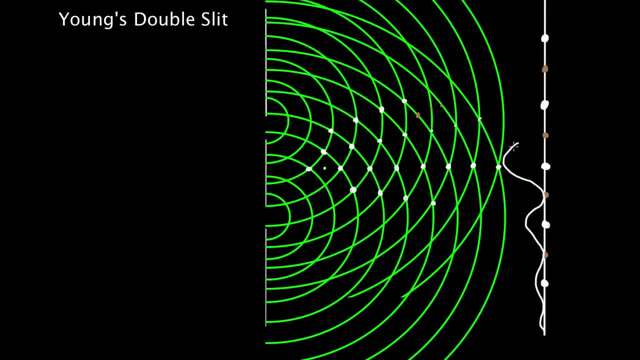 They get weaker and weaker as you go out. At some point it's hard to see. Same on this side: 0, bright spot. 0, bright spot. This is the classic double-slip pattern you'll see on the wall. 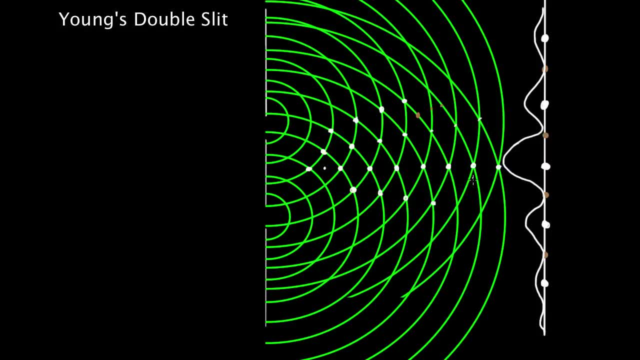 And it's caused by wave interference in two dimensions. And what's the rule for wave interference in two dimensions? This is the same rule as the wave interference for one dimension. It was this, Remember, for one dimension: delta x, the path length difference. 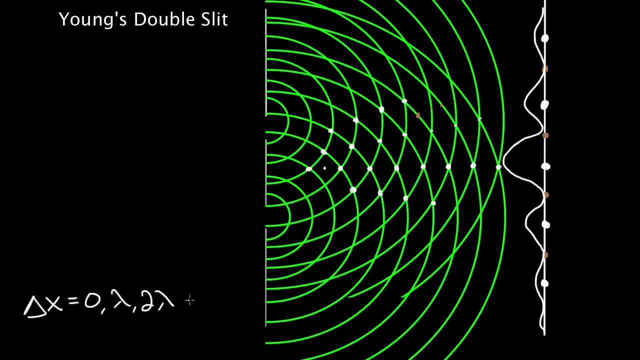 had to be 0, lambda, 2 lambda, 3 lambda, so on, would give us constructive interference. And now, if you're paying close attention, you might say: hold on, there was a condition, Remember this was only true if there was no funny. 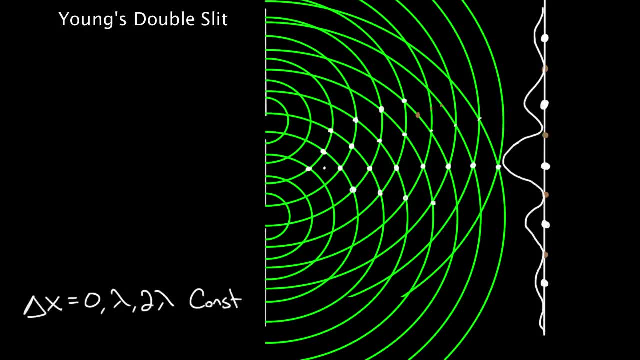 switcheroo business with the back of the speaker. We had to make sure that these two sources were in phase to start off with. Is that true of these light waves? It is, In fact. that's why we do it double-slip like this. 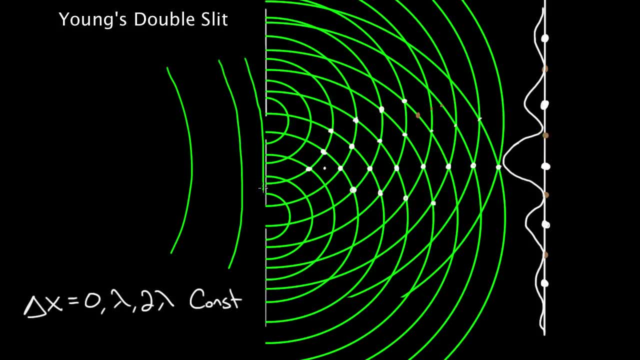 That's why we take one wave, We let one wave come through here. That way we break it up into two pieces. Why? Because we know if a peak was going into the top hole, well the same wave was going into the bottom hole. 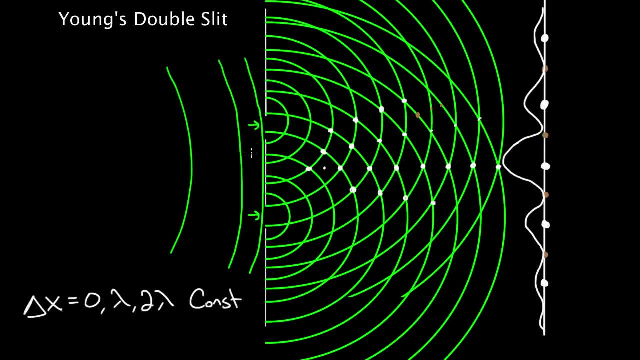 That's also a peak. This is a tricky wave. A quick, easy way to make sure your two sources coming out of these two holes are exactly in phase. You don't have to worry about any phase difference caused by the source. You just have to worry about a phase difference caused. 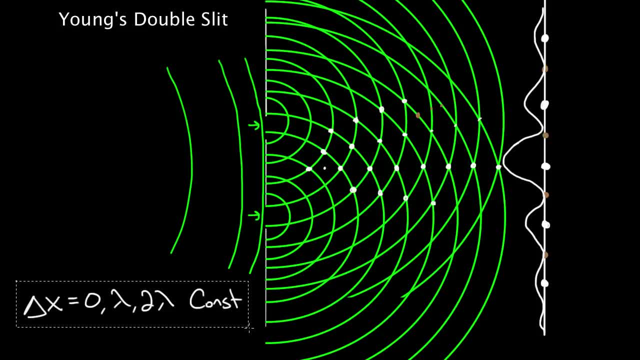 by the fact that these waves are going to travel different distances to different points. And what do I mean by this? What does path length difference mean here? Well, if I look at it from this top line, or this top hole, this is basically like our speaker. 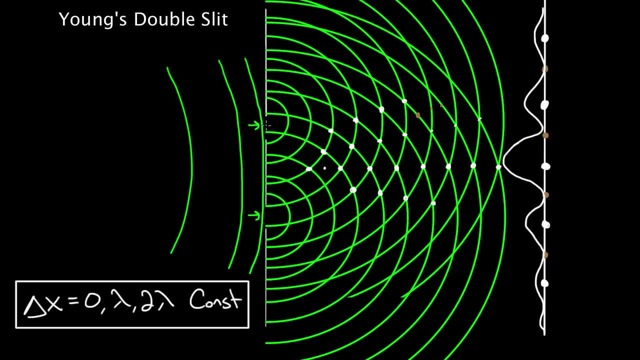 One source here. one source here, but it's light instead of sound waves. From here to the center bright spot, the wave from the top hole had to travel a certain distance, And from the bottom hole to that spot, wave had to travel a certain distance. 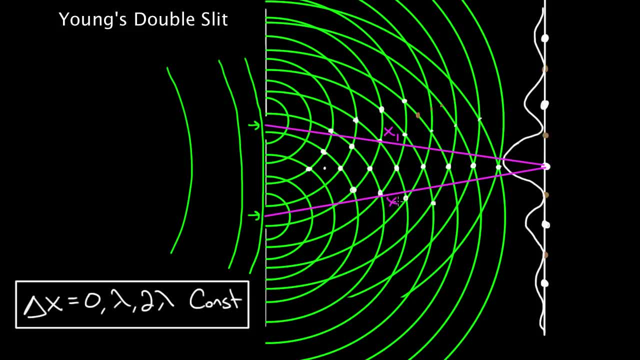 So basically this we can call x1, this length x2.. And the path length difference would be x1 minus x2.. The difference in these- and you can just make it the absolute value if you want, but the size of the difference. 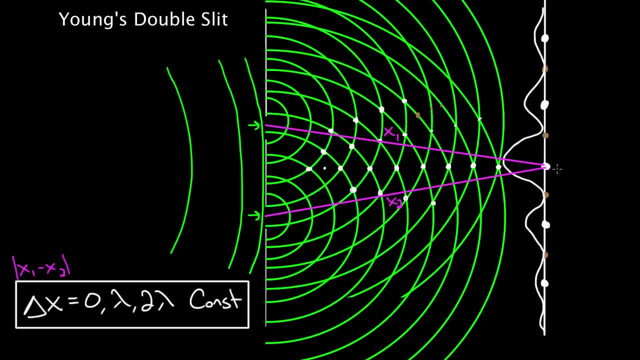 between these two path lengths. What is that going to be for? right in the center? Well, that one's just. delta x equals 0. Right, Because the waves are traveling the same distance to get to that point, And that makes sense. 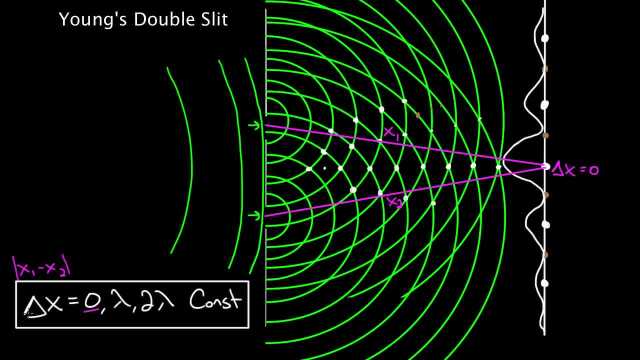 That's a constructive point, because 0 gives you a constructive point when the path length difference is 0.. How about the next point? Well, the wave from the bottom has to travel this far. The wave from the top hole has to travel this far. 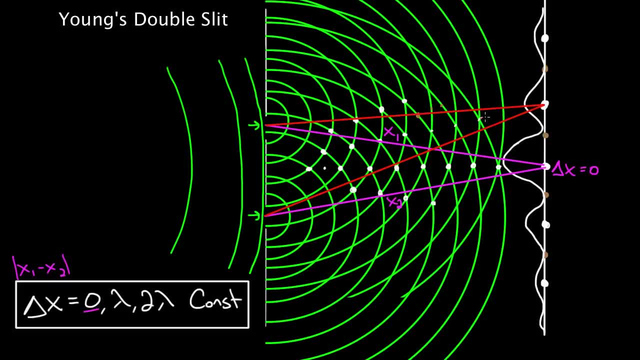 This time they're not traveling the same distance. The wave from the bottom hole is traveling farther. How much farther? Well, it's got to be the next one, It's got to be lambda. So this wave is going to be traveling. 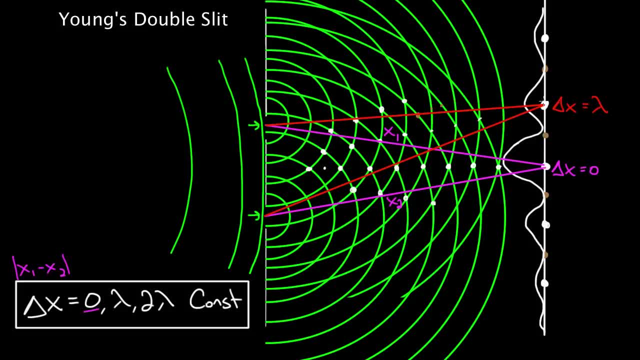 The bottom wave would travel one wavelength further to get to this point than the wave from the top hole, because that's the next possibility for constructive interference. Note: it's not from here to there, that's one wavelength. This is a common misconception. This distance on the wall between constructive points. 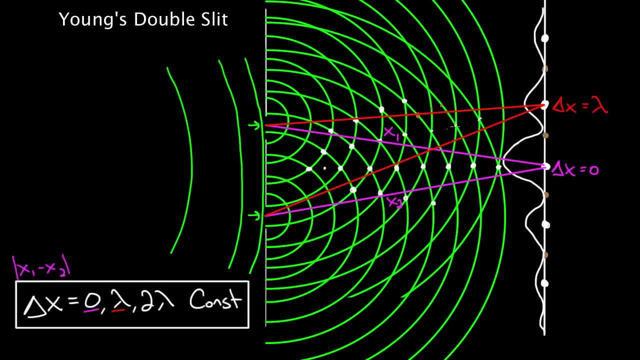 is not one wavelength. The difference in path length that one wave travels to get there compared to the other wave is one wavelength. And I bet you can guess the next one. The next one, delta x, would just be two wavelength. And you can keep going. 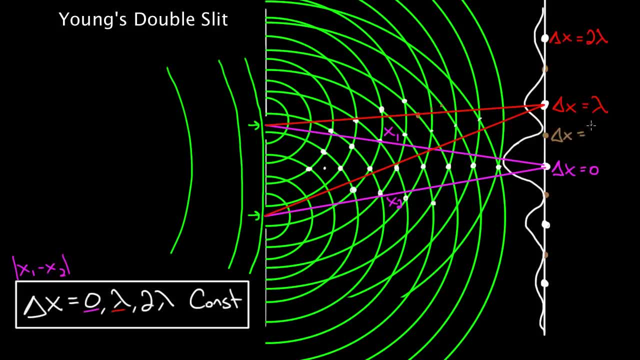 How about the destructive points Shoot. you know how to do that. These are going to be the half wavelengths lambda over 2.. This one's going to be 3 lambda over 2, and so on And down here. what would you get? 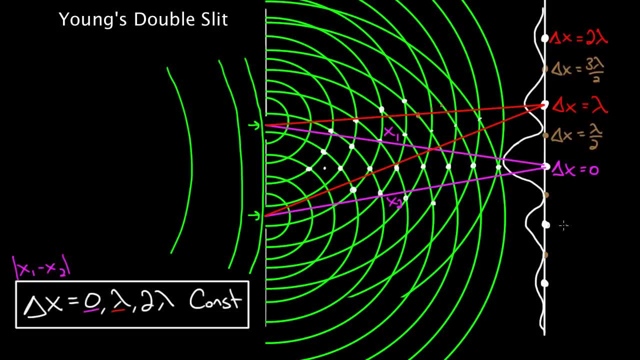 Well, if you got rid of the absolute value sign- and you wanted to- you could start talking about this. delta x would be negative- 1 lambda, This one would be negative, 2 lambda, and so on. So you could have negative values if you wanted to denote the fact that that might be lower. or higher, depending on where you were in this interference pattern.